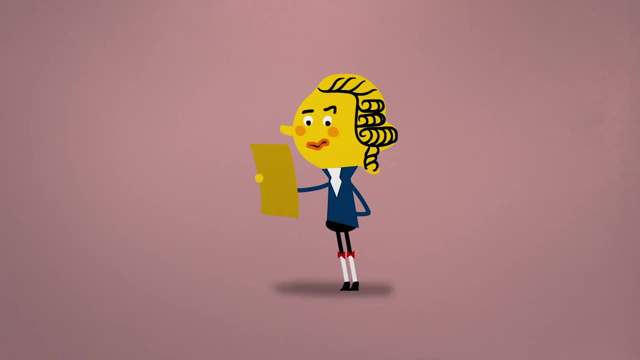 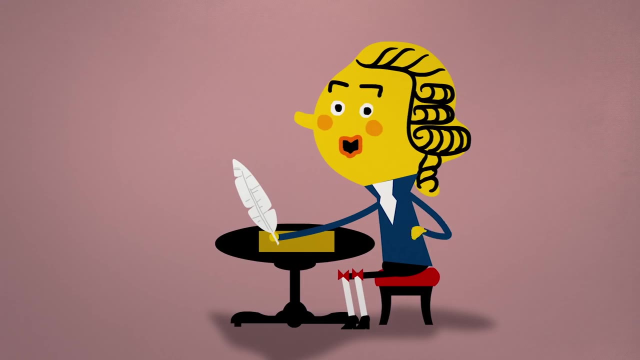 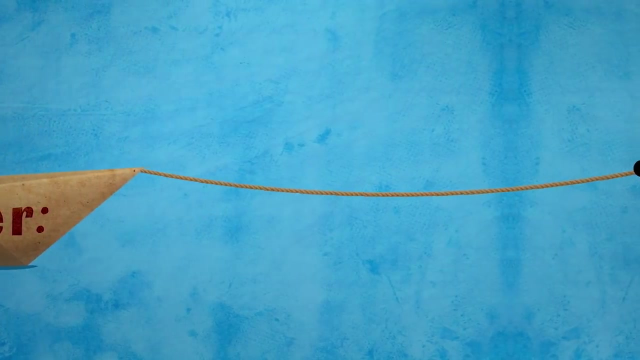 Carl wrote to Euler for help with the problem. Euler first dismissed the question as having nothing to do with math, But the more he wrestled with it, the more it seemed there might be something there after all. The answer he came up with had to do with a type of geometry that did not quite exist yet. 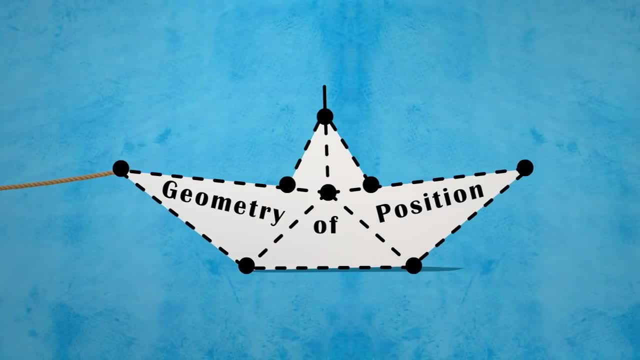 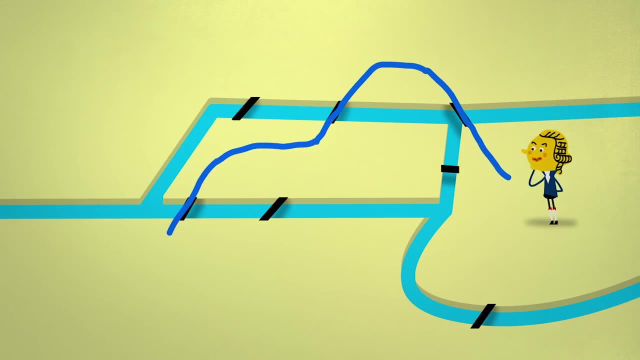 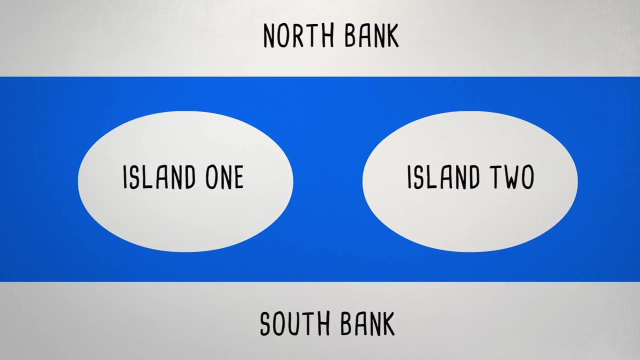 what he called the geometry of position, now known as graph theory. Euler's first insight was that the route taken between entering an island or a riverbank and leaving it didn't actually matter. Thus, the map could be simplified, with each of the four landmasses represented as a single point. 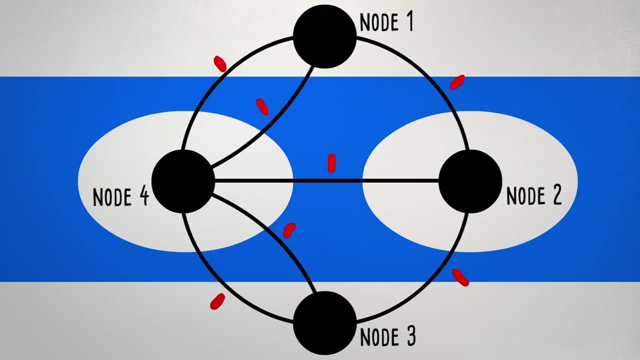 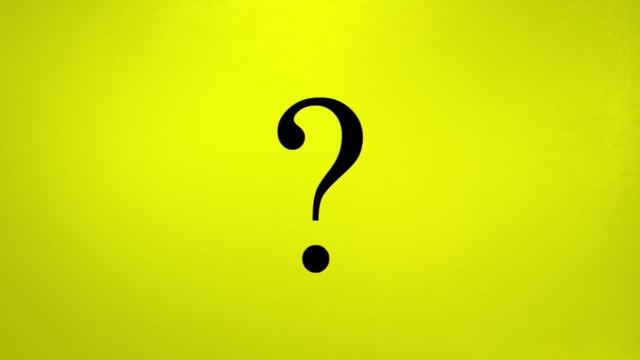 what we now call a node, With lines or edges between them to represent the bridges, And this simplified graph allows us to easily count the degrees of each node, That's the number of bridges each landmass touches. Why do the degrees matter? 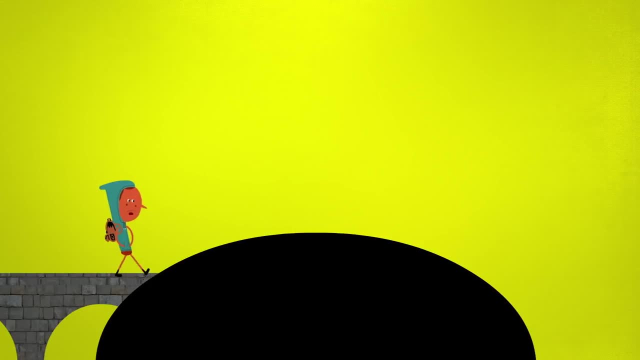 Well, according to the rules of the challenge, once travelers arrive onto a landmass by one bridge, they would have to leave it via a different bridge. In other words, the bridges leading to and from each node on any route must be the same. 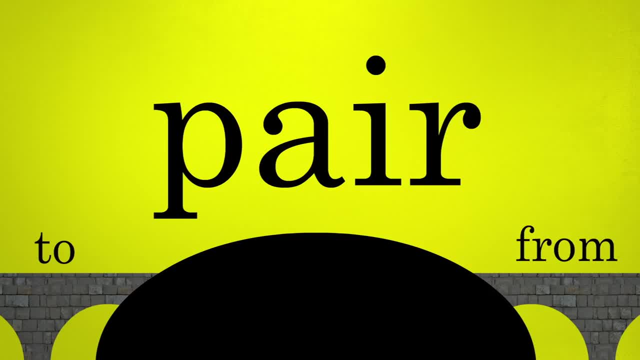 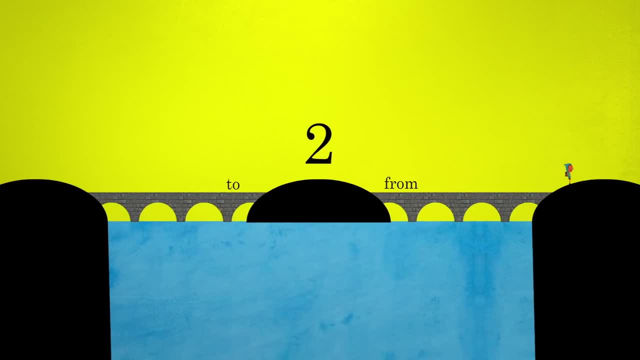 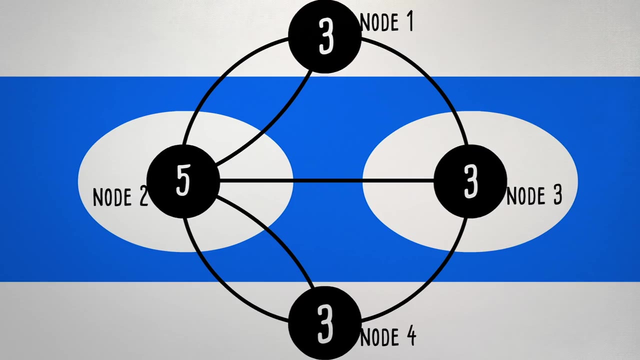 They must occur in distinct pairs, meaning that the number of bridges touching each landmass visited must be even. The only possible exceptions would be the locations of the beginning and end of the walk. Looking at the graph, it becomes apparent that all four nodes have an odd degree. 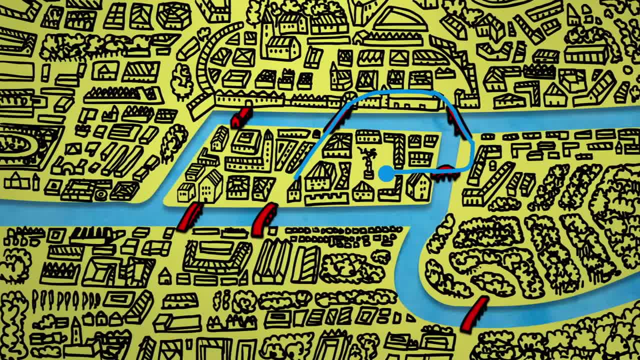 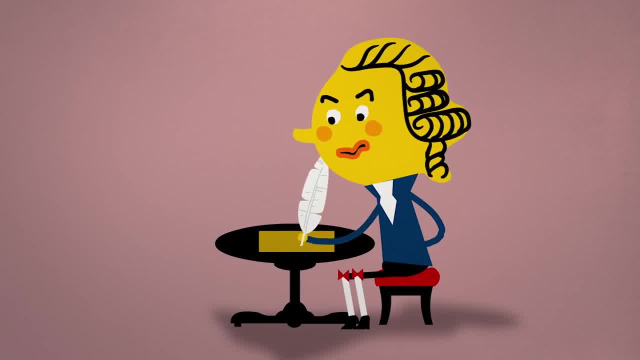 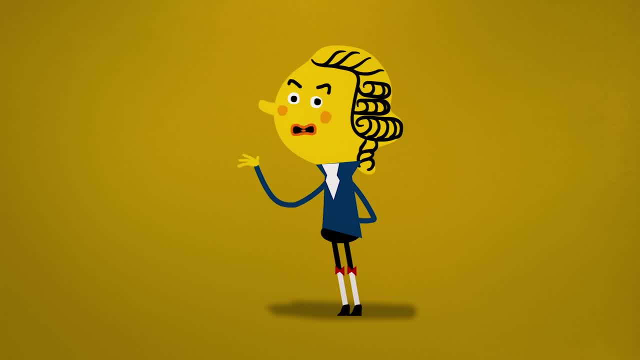 So, no matter which path is chosen, at some point a bridge will have to be crossed twice. Euler used this proof to formulate a general theory that applies to all graphs with two or more nodes: A Eulerian path that visits each edge only once. 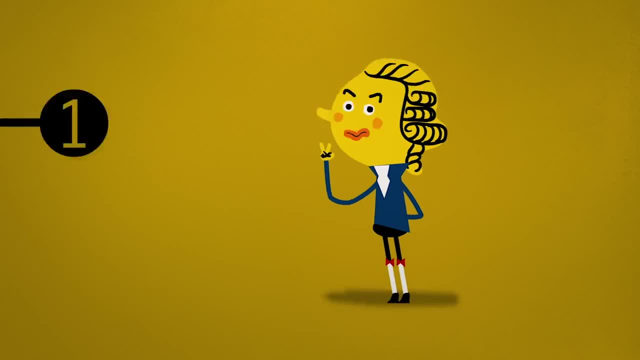 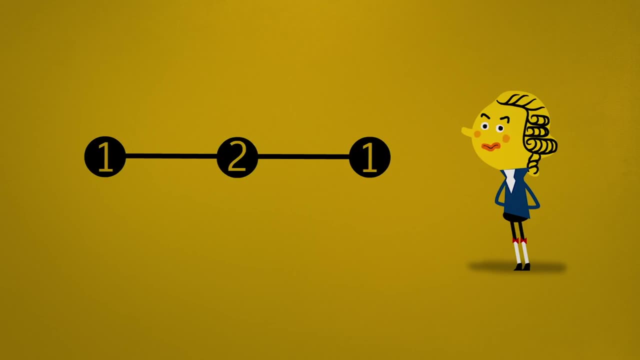 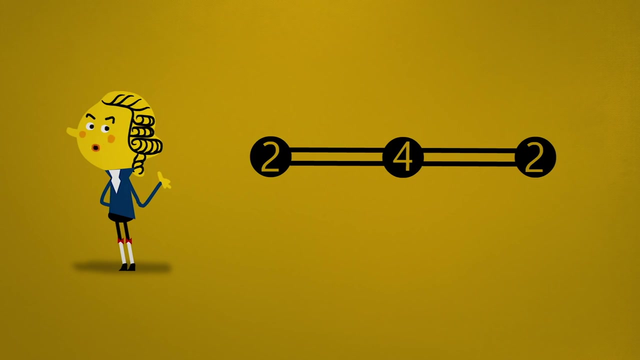 is only possible in one of two scenarios. The first is when there are exactly two nodes of odd degree, meaning all the rest are even There. the starting point is one of the odd nodes and the endpoint is the other. The second is when all the nodes are of even degree. 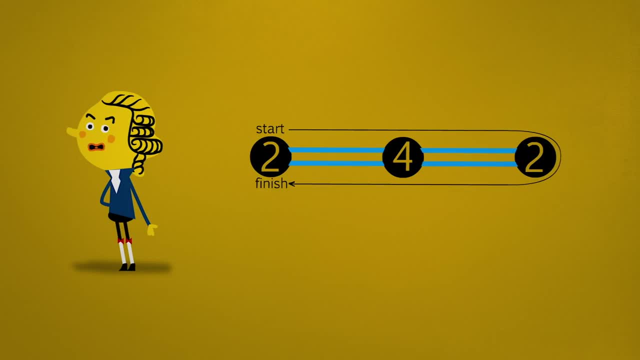 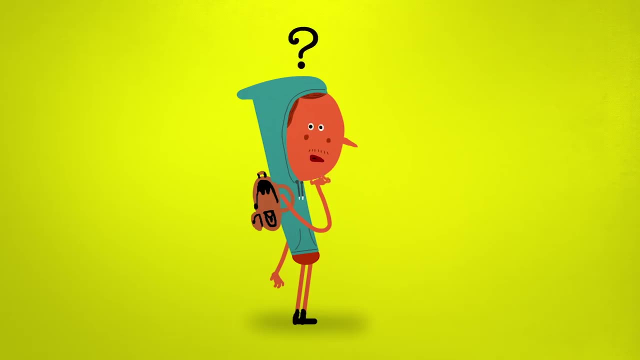 Then the Eulerian path will start and stop in the same location, which also makes it something called a Eulerian circuit. So how might you create a Eulerian path in Konigsberg? It's simple: Just remove any one bridge And it turns out.